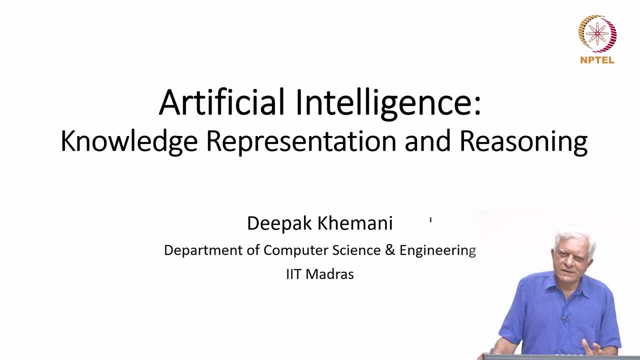 course. Now, this course is, as the title suggests, focuses on one of the key aspects of artificial intelligence, which is: how do agents know their environment, the domain and, as they acquire more knowledge, as they get more information, how do they reason with what they know? 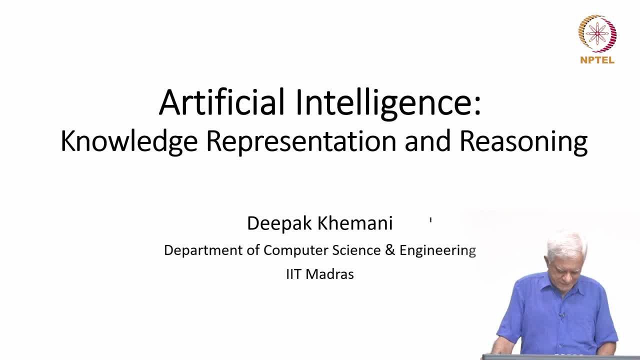 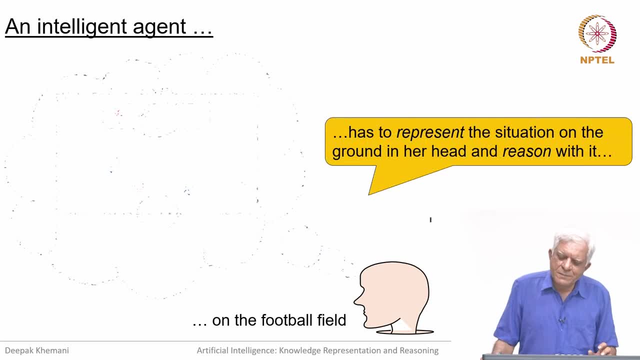 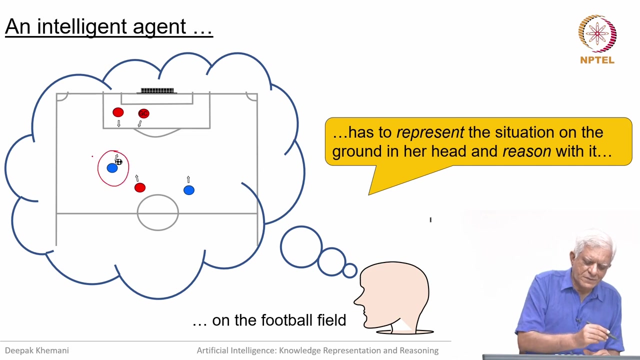 So our course is going to be focused on that. So think of an intelligent agent on a football field. That player has to represent the situation that she is in and has to reason with that situation. So, for example, if this is the player that you are talking about, 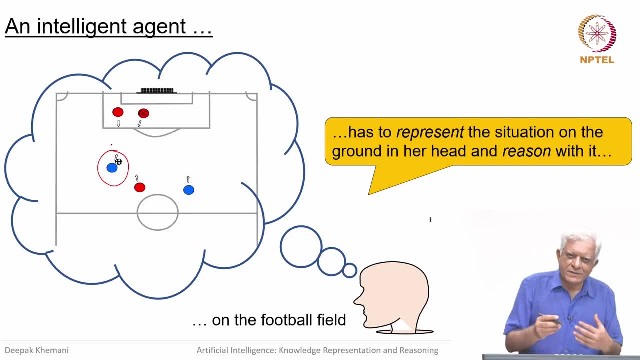 the player is running towards the goal, but the other opposing players are moving towards her. The opposing team is a red team, but her partner is also moving forward. So what should she do? She has to be aware of the situation and reason about what is happening. 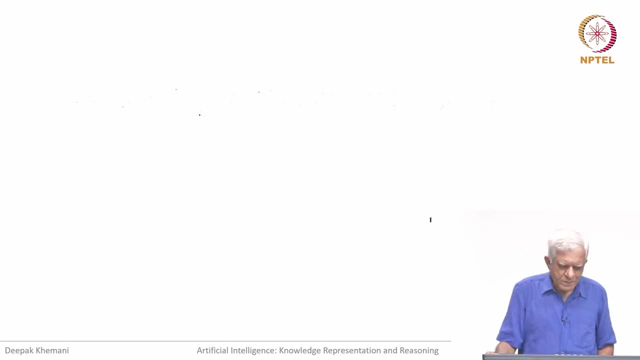 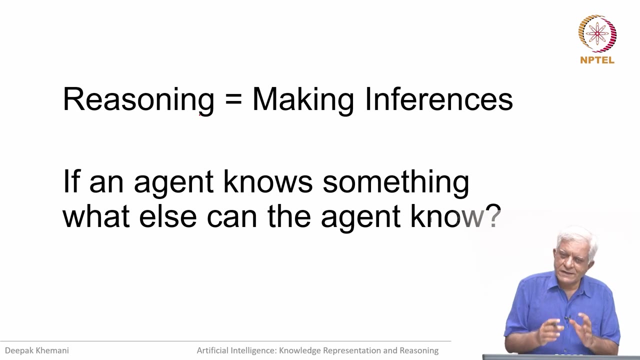 and, of course, make her plans. Reasoning: when we say reasoning, we say making influence. You know something. what else can you know? essentially, What are the inferences that you can make? And our course is going to be focused on both these things. How do you know something? How? 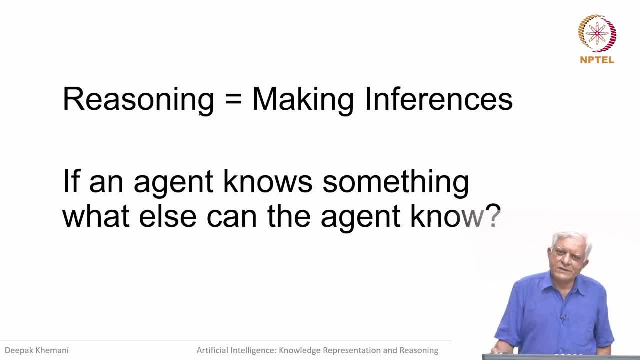 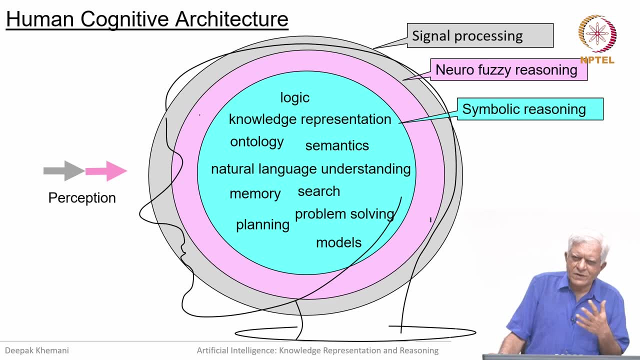 do you represent something And, as a consequence, what else do you infer? Now, if you look at the human cognitive architecture, we can think of it as a three-layered architecture. The outermost layer, shown in gray here, does signal processing. So we see with our eyes. 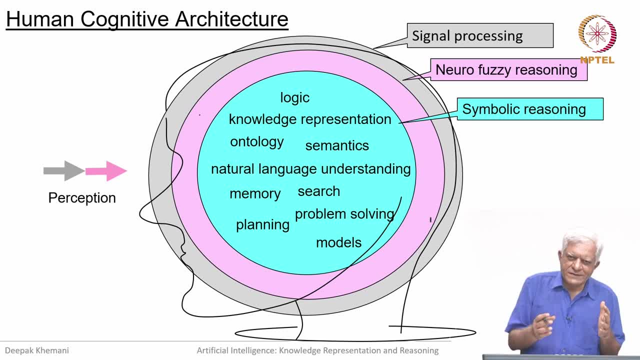 we hear from with our ears and so on, And it processes signals. Then there is a next layer, which is the neurophysiology. This is the layer which converts signals into symbols, And in our course, we are interested in symbols, and not only in symbols but in reasoning with symbols, essentially. So we 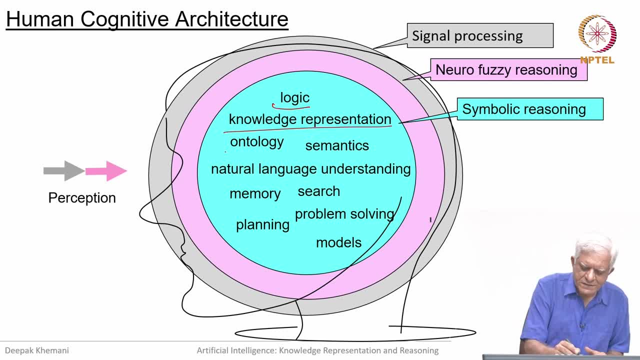 will cover topics like logic, knowledge, representation, ontology, semantics, a little bit of natural language understanding, but not too much more, And the other topics I cover in some other courses, such as search methods and so on. So let us get started. 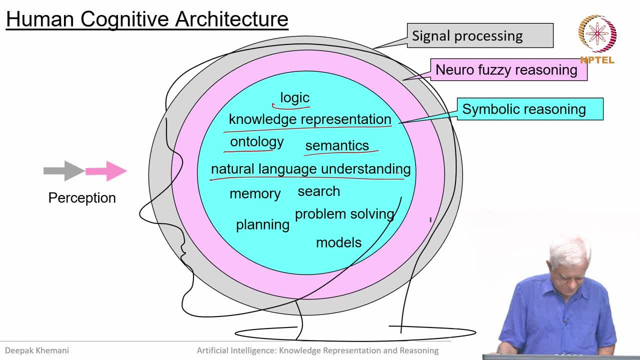 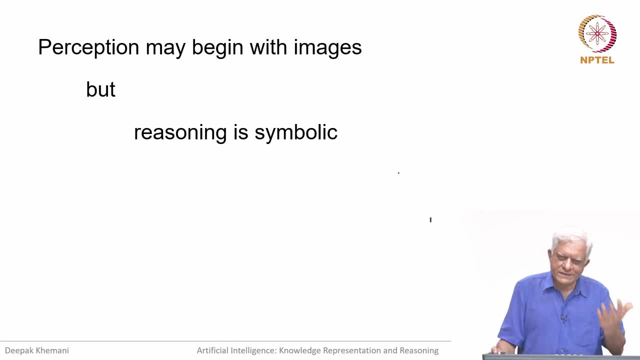 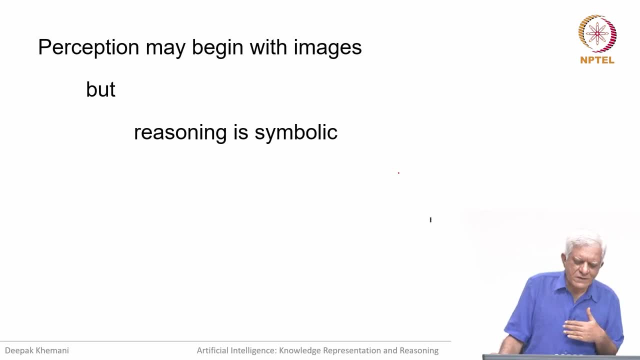 converts them into signals. The fuzzy system converts it into a signal, But reasoning itself is symbolic And our focus is going to be on reasoning. eventually We investigate the algorithms for reasoning on symbolic representations. We are going to focus instead more on for some time. 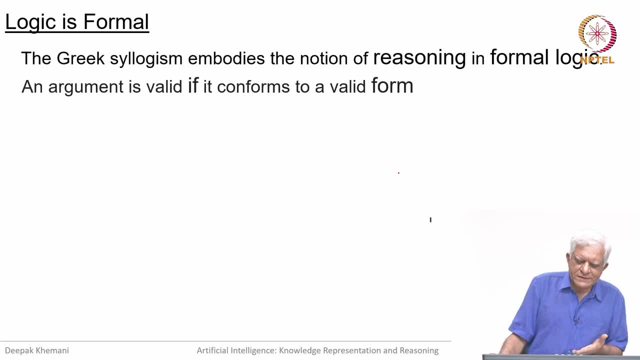 So we start on logic, and one of the oldest things that we know of logic is the Greek syllogism, which embodies the essence of logic. and the essence of logic is that reasoning is formal, that reasoning is valid, or arguments are valid if they conform to a valid form. 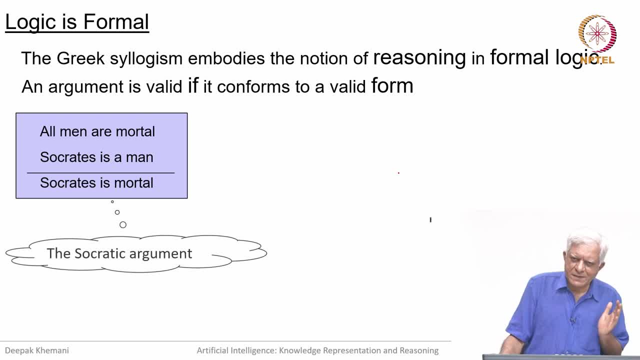 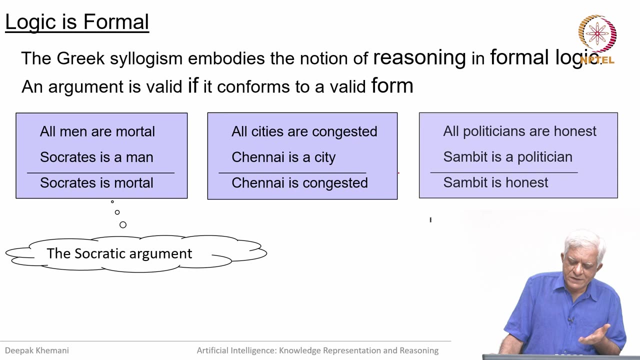 They are not so much concerned with content. So this is a standard example that we talk about very often. all men are mortal. Socrates is a man and therefore Socrates is mortal. let us call the Socratic argument, But you can see that it is a form that is important. 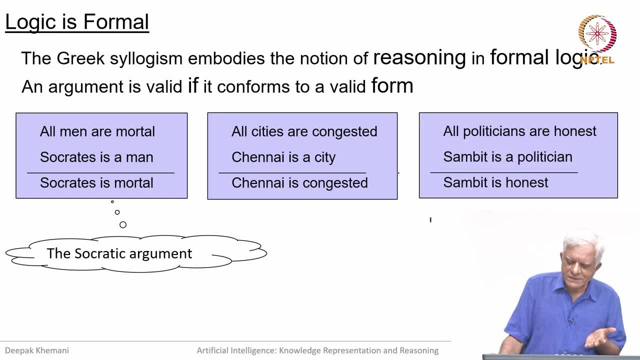 You can say: all cities are congested, Chennai is a city and Chennai is congested. All politicians are honest. Sambit is a politician. Sambit is honest. As long as the argument has a valid form, then if the premises are true, then the conclusions. 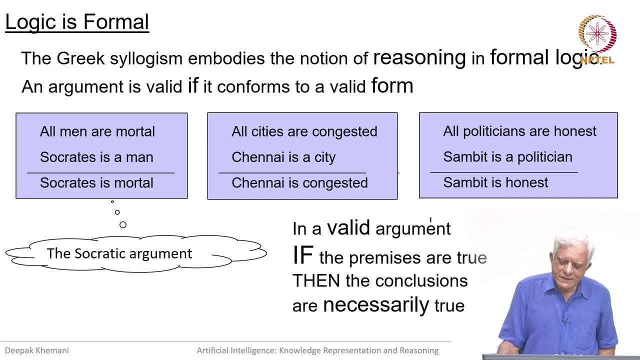 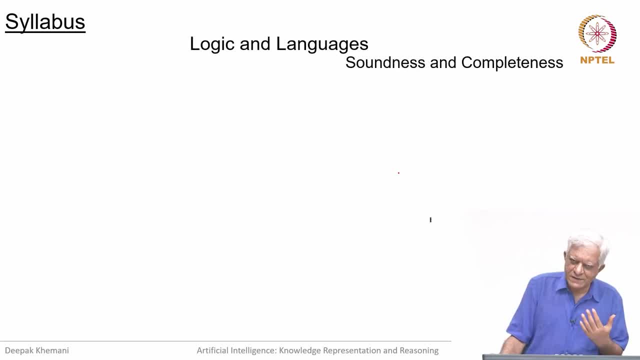 will necessarily be true. That is the key idea behind logical deduction, The syllabus that we will cover in this course. we will start with introducing logic and the fact that we represent things symbolically. we will talk about soundness and completeness. We will start with the simplest of all logic, which is proportional logic, and study some. 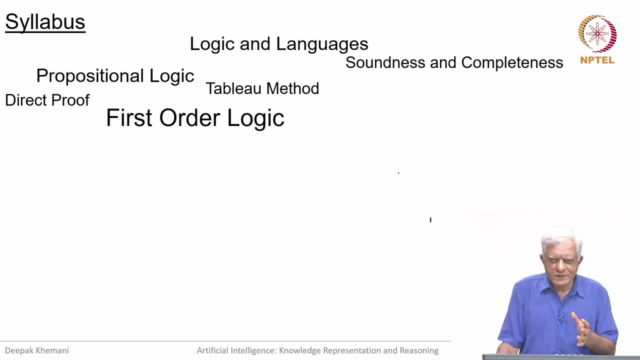 proof methods, the direct proof and the tableau method. before we move on to the main part of our course, which is going to be on first order, logic, Where we will look at algorithms, Algorithms like forward chaining, backward chaining, the resolution method. We look at their connection to the idea of logic programming, declarative programming. 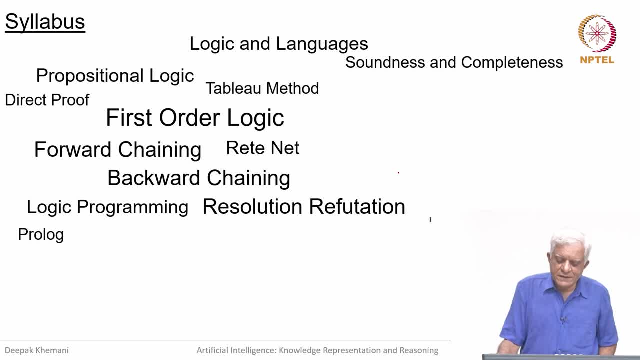 An example will be prologue and we will also look at forward chaining as a declarative language using the retinit. Then we will move on to representation, in which we will look at the idea of reification, which is the idea of creating concepts in your head.